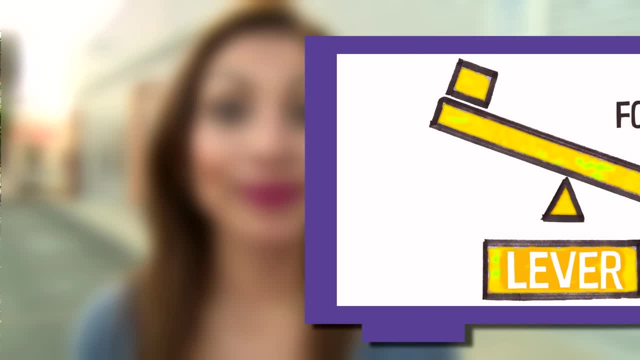 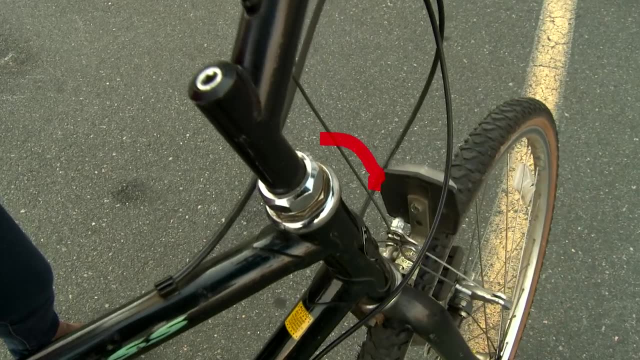 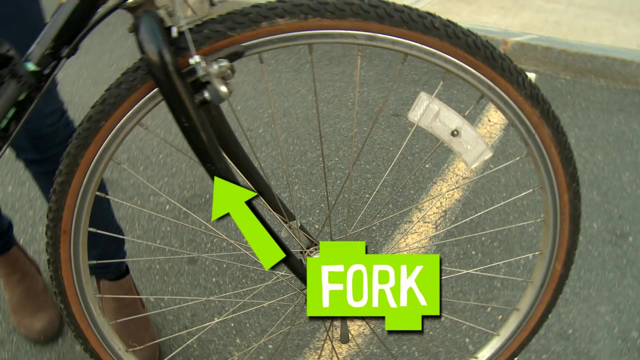 moves a load on one end. when a force is applied to the other end, The handlebar is actually a lever. When I move the handlebar it pivots right here, which makes it very easy to turn the wheel. It would be really hard to turn the wheel at the fork if you didn't have handlebars. 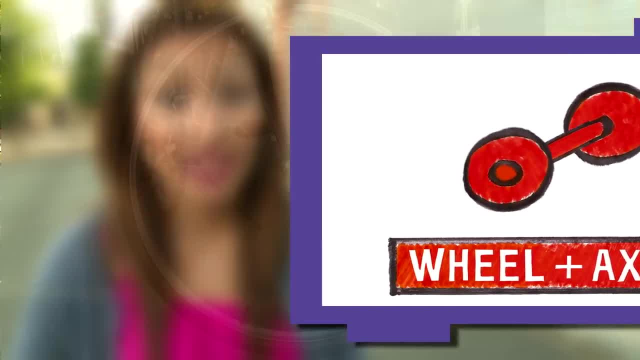 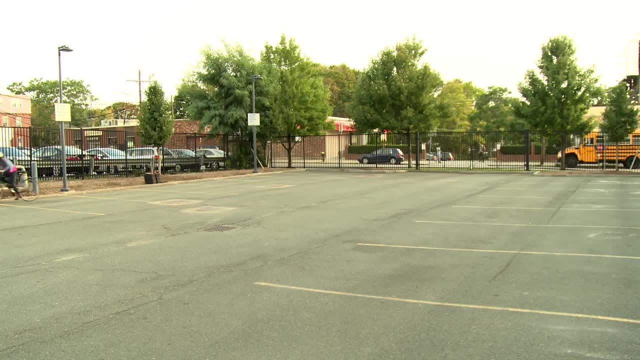 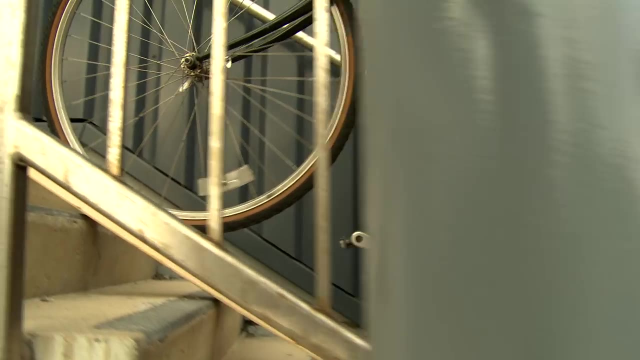 The next simple machine is the wheel and axle. Here's the wheel. It spins on this rod called an axle. Wheels can help carry heavy loads around for long distances. The incline plane is another type of a simple machine. It is a ramp, an angled surface that helps you move. 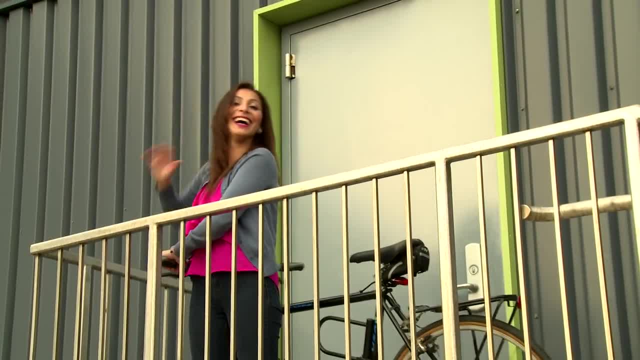 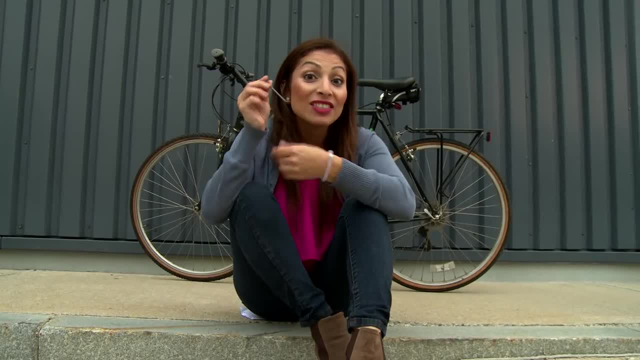 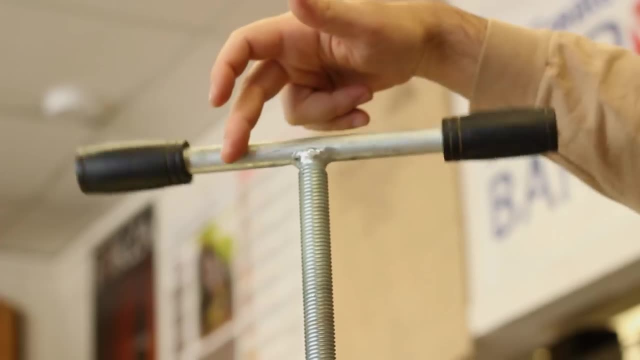 objects up and down a height Ta-da. The incline plane made it much easier for me to take my bike up the stairs. Another type of simple machine is the screw. A screw is actually another incline plane, wrapped around a pole in a spiral shape. Screws can convert a force. 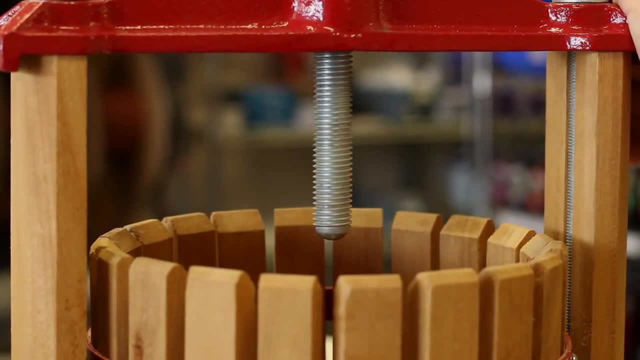 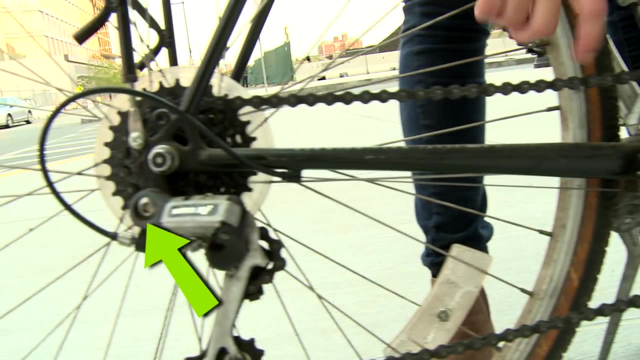 that goes around and around into a force that goes up and down, like with this press that gets juice out of apples. There are screws all over this bike holding the different parts of the bike together, And this chain wheel is a nice example of another simple machine. 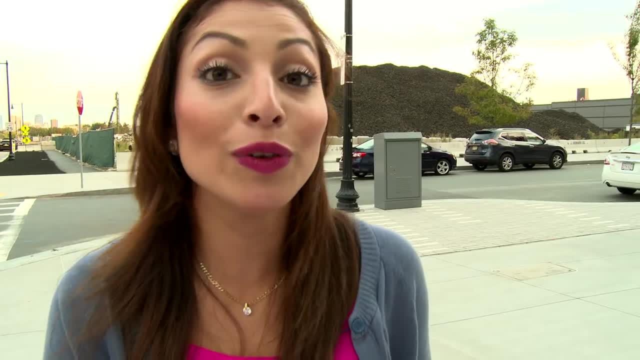 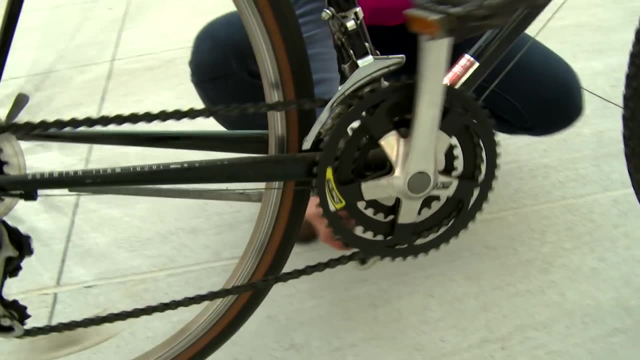 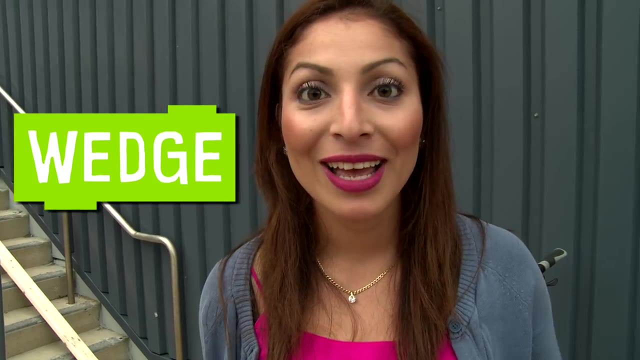 A pulley. A pulley is a wheel on an axle that moves things and changes the direction of a push or a pull. When you push down on the pedal, the front wheel moves the chain, which then turns the rear wheel and moves the bike forward, And the final simple machine is a wedge A. 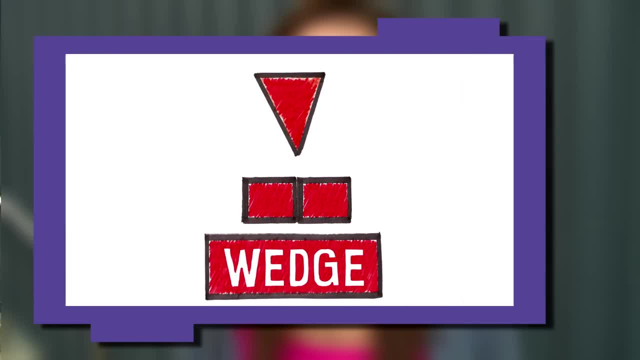 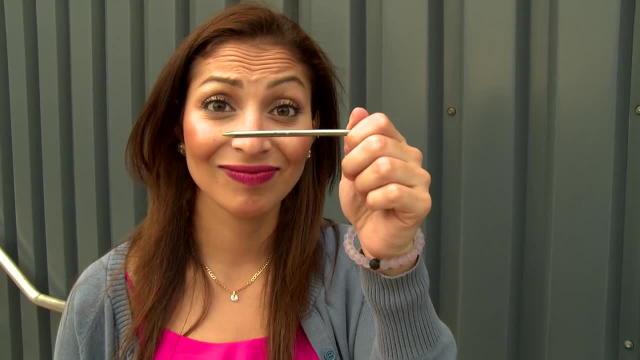 wedge is two inclined planes put back to back. You can use a wedge to push two objects apart. The kind of wedge that I don't want in my bike is this nail, especially not in my tire. A nail would spread apart the rubber material in my tire and make a hole. 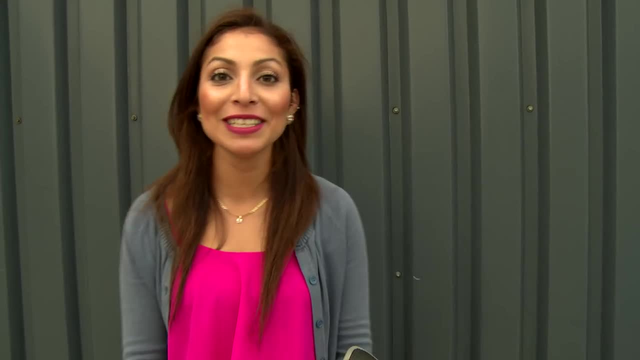 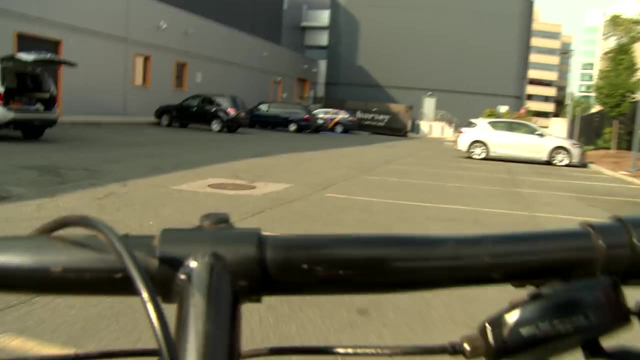 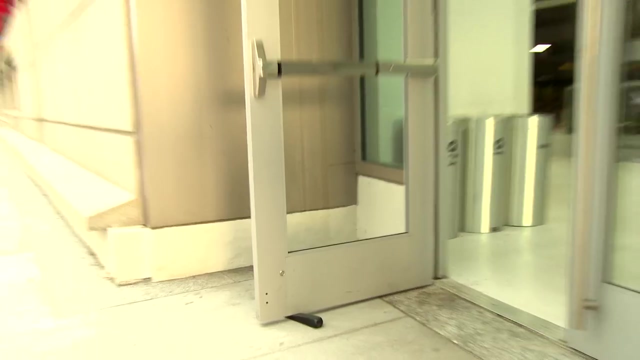 Okay, now that we know about simple machines, let's see if we can find some out in the real world. And maybe we can find all six. There's a wedge. See this wedge keeps this big door open. Let's see what else we can.